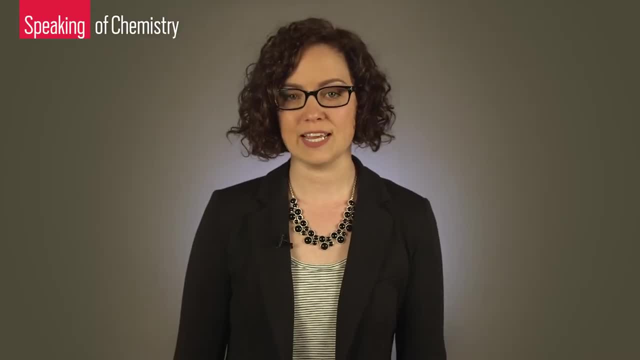 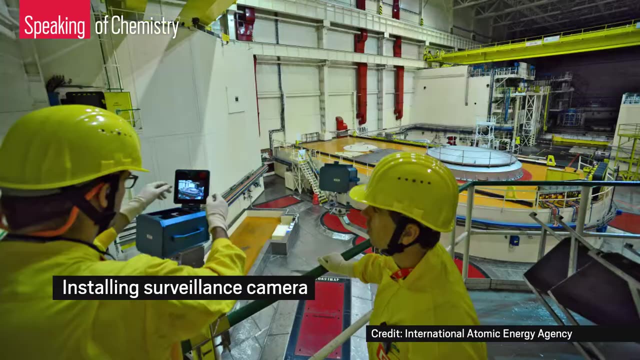 So how can you ensure that this material is being used only for peaceful purposes, like power generation, and not for building a bomb? International inspectors use tools like isotope identification devices, surveillance cameras and special seals that prevent unauthorized access to monitor weapons-grade materials. 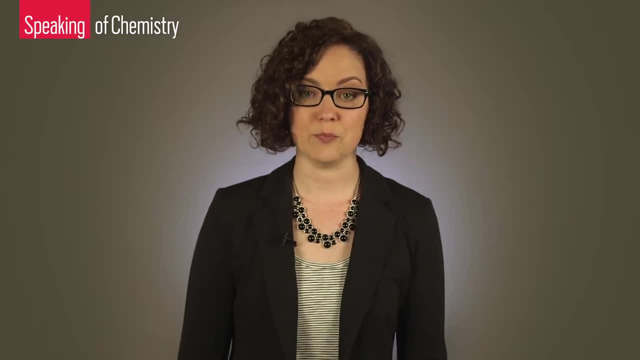 that ought not go missing. Sometimes, however, material does escape regulatory control. Often it's simply mishandled, but it could also be stolen or intentionally diverted. If radioactive material is found somewhere it's not expected, nuclear forensic scientists can help identify the material where it came. 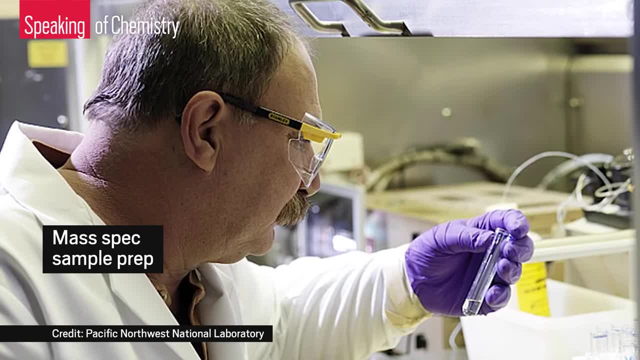 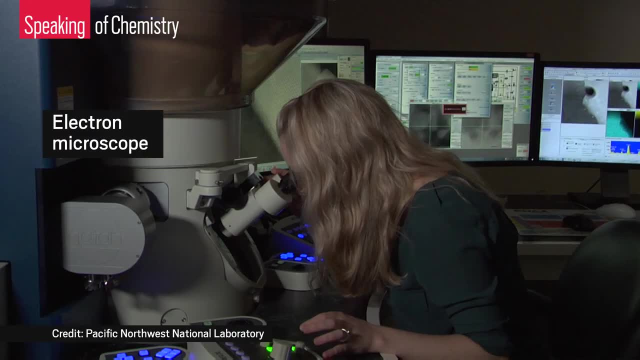 from and whether it was used for illicit activity. These scientists have a host of techniques and tools at their disposal to understand the chemical makeup of a given material, like high-precision mass spectrometry to characterize its isotopic content, or electron microscopes. 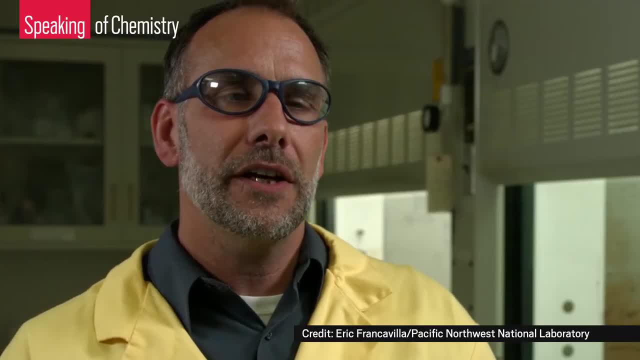 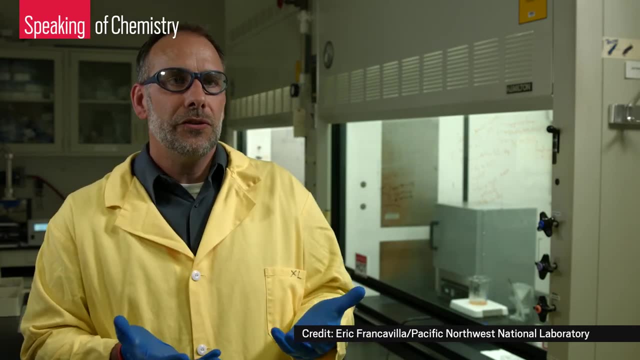 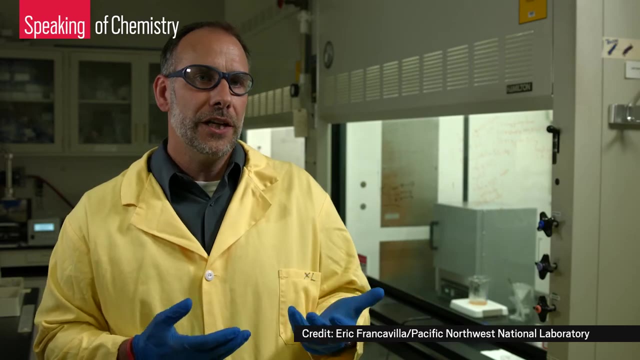 to characterize the material's physical properties. It could be as simple as looking at the physical form of the material, And then, beyond that, we can get more detailed, Not unlike what forensic chemists do in a traditional sense. but we can look in more depth and look at the grain structure. 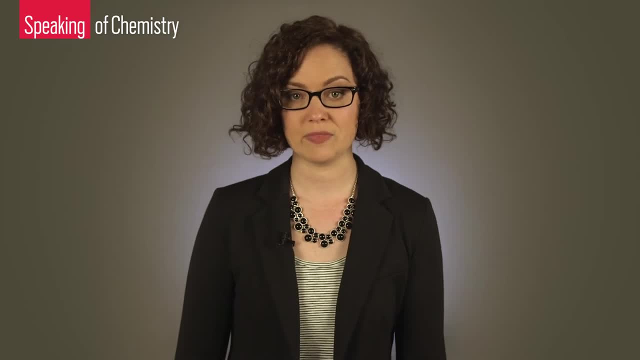 John Schwantes is a nuclear forensic scientist at Pacific Northwest National Laboratory. He told me that, although these analytical tools are helpful to officials investigating a case that found radioactive materials, there's still work to do. The nuclear forensics community is currently working to better analyze and 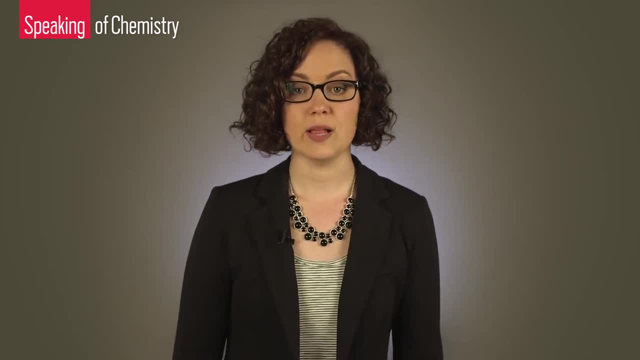 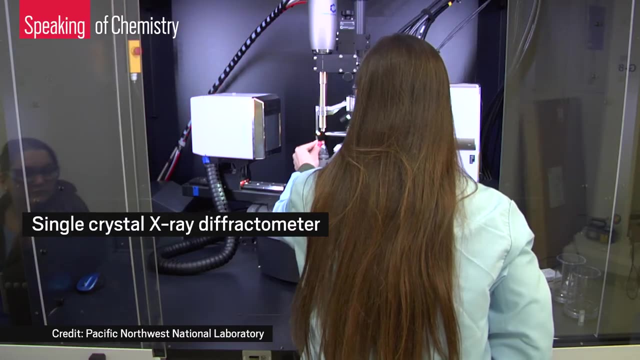 understand the trace elements that appear in nuclear materials, as well as develop tools that could reveal which reagents were used to process a material. We're not going to be the smoking gun that solves the case. We're going to be a small piece in a larger investigation. 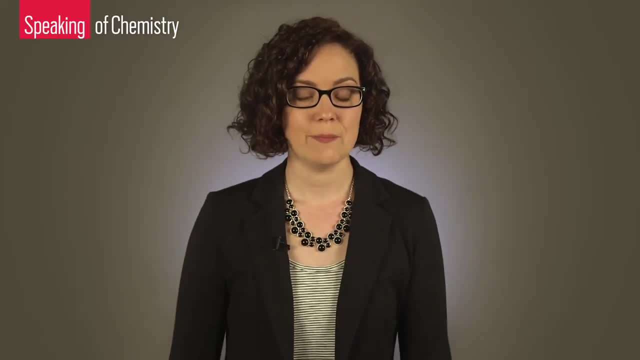 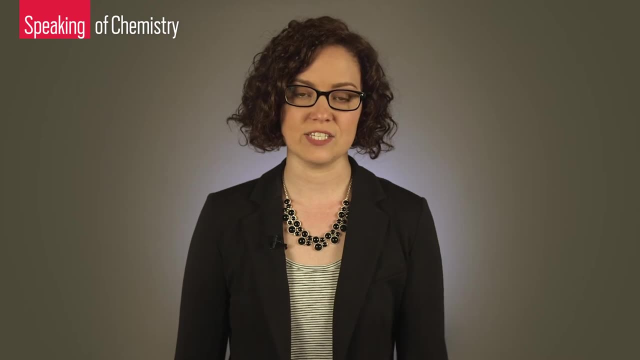 Schwantes works with material that is already in law enforcement's control, But international inspectors don't always have direct access to nuclear materials and operations, such as when a country is not granted access to its facilities, In those cases, being able to monitor nuclear activity. 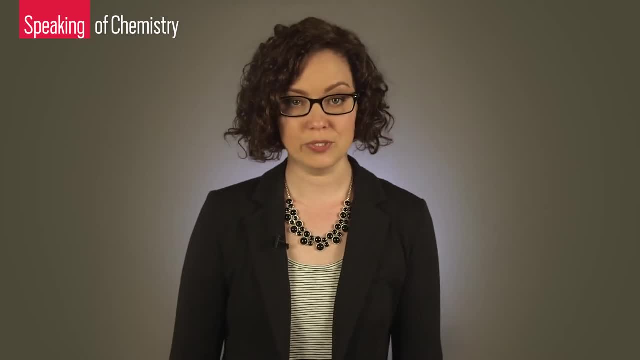 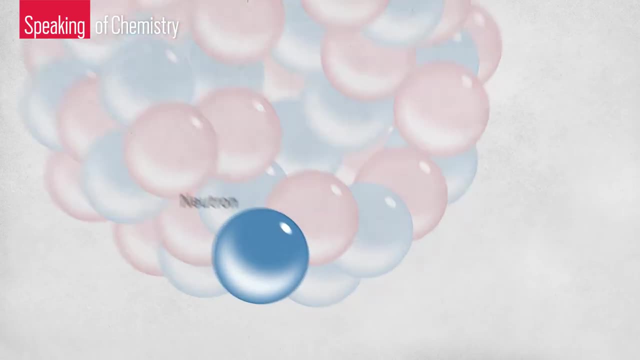 remotely, say from several kilometers away, would be a valuable tool. We spoke with researchers at Lawrence Livermore National Laboratory and Brookhaven National Laboratory. We're developing technology that senses subatomic particles called antineutrinos, which nuclear reactors emit as part of the fission process. 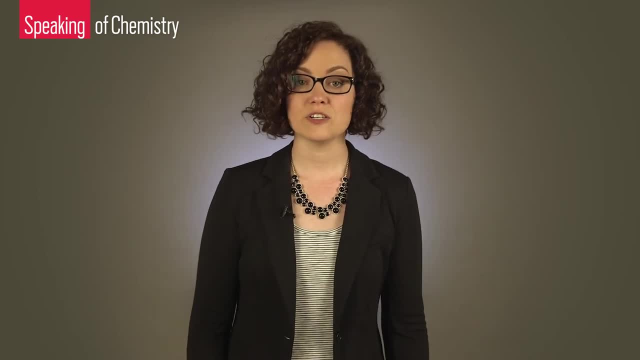 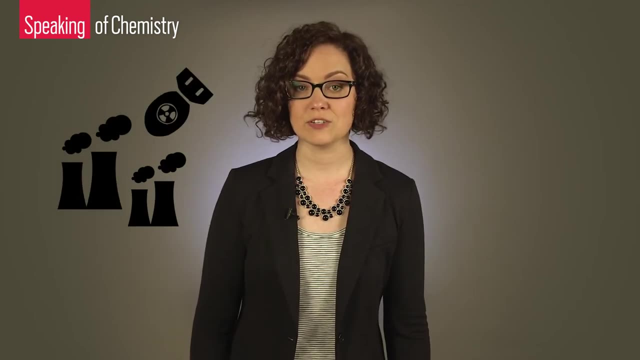 The detector, which is called WATCHMAN, could be used to monitor a large swath of territory and potentially pinpoint reactors making plutonium for weapons use, even if they were hidden among known reactors used to generate power. So you essentially account for the known reactors and you say: ah wait, there's this extra little. 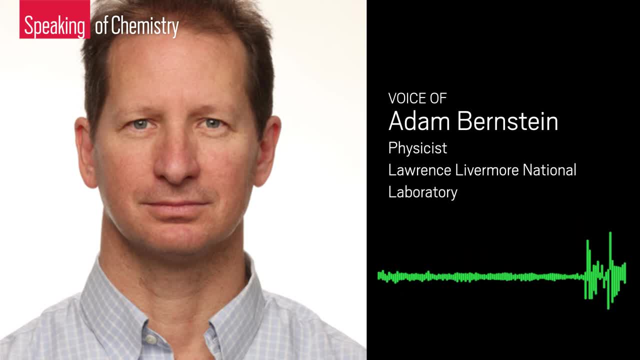 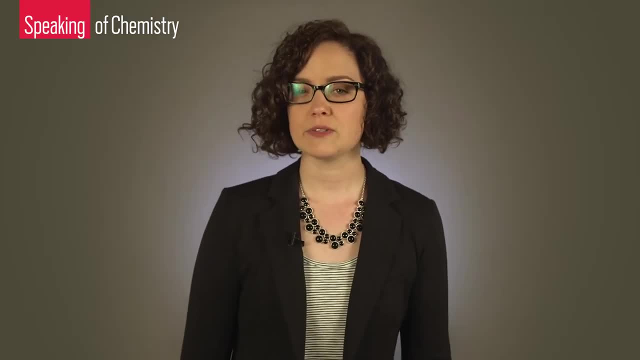 bright spot of extra antineutrinos that must be coming from an additional production capability. Adam Bernstein leads the WATCHMAN project, which is currently under construction. Antineutrinos are very hard to detect and in order to pick up signals from tens or hundreds of kilometers. 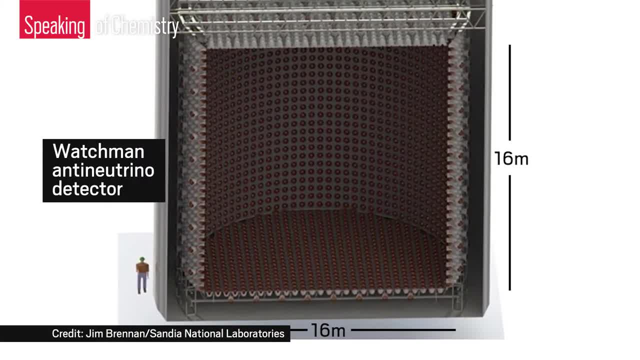 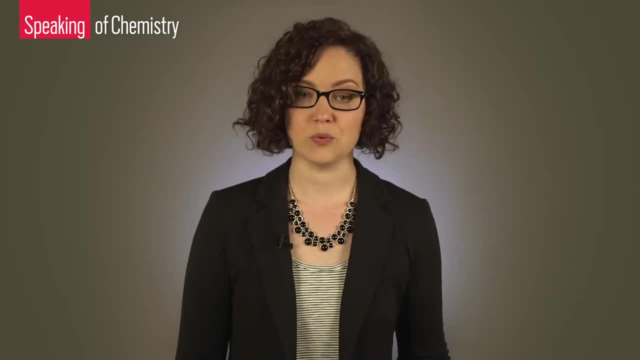 away. the WATCHMAN team will need a very sensitive, very large detector. So the current design is massive, roughly 16 meters tall and 16 meters in diameter. The first generation detector will be filled with water, doped with a little gadolinium and it'll sense Cherenkov radiation. 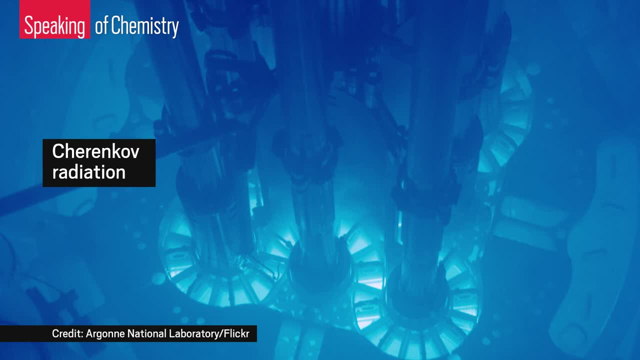 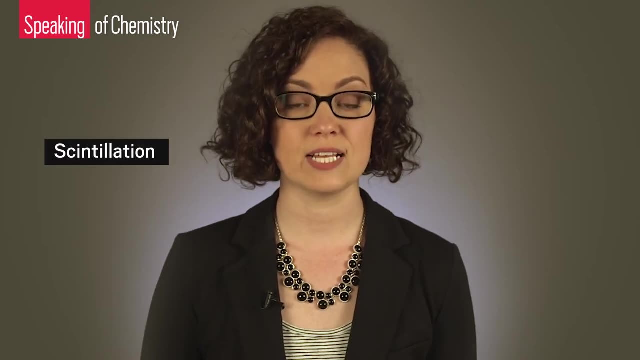 which you might recognize as the characteristic blue glow of an underwater nuclear reactor. But you can also detect antineutrinos using something called scintillation. In this situation, particles collide with organic molecules and generate a flash of light And a future generation. 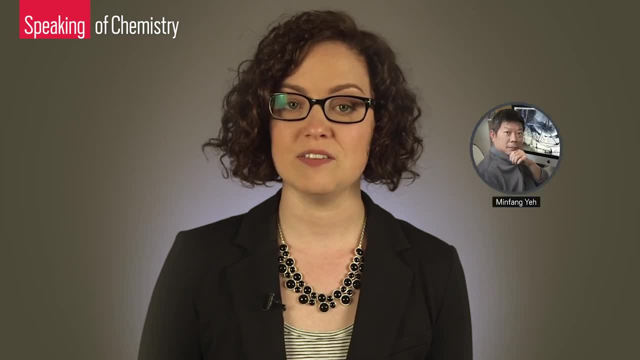 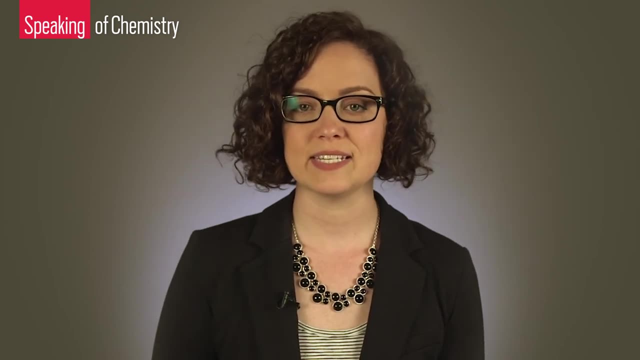 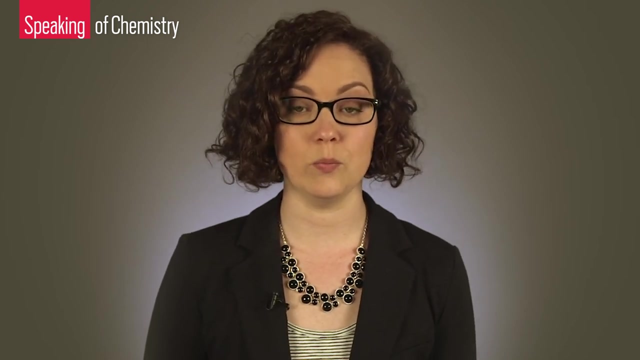 of WATCHMAN will combine those two detection methods. Team chemist Minfang Yeh tells us the dual-band detection of the water bath combined with just a little bit of organic scintillator liquid would enable scientists to better separate interesting signals from background noise. Yeh said the challenge was finding a way to mix the scintillator liquid. 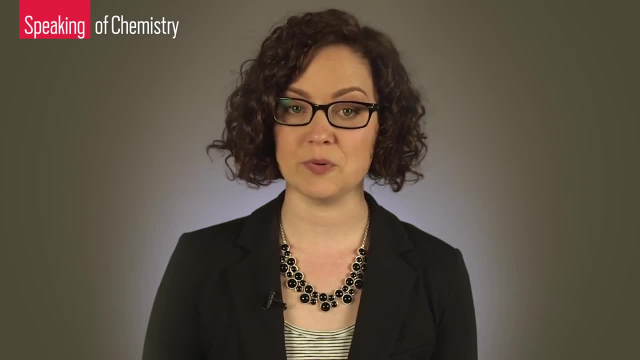 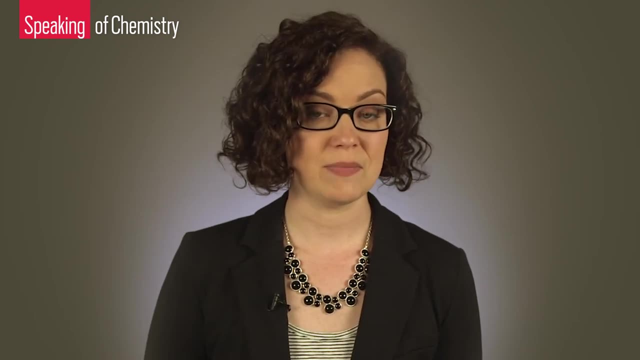 with the water and some other necessary additives, without the mixture separating or becoming cloudy, which would interfere with the transmission of the antineutrinos. He also needed the liquid to be eco-friendly and mass-producible. His team experimented with several formulations before finding a potion capable of generating both Cherenkov. 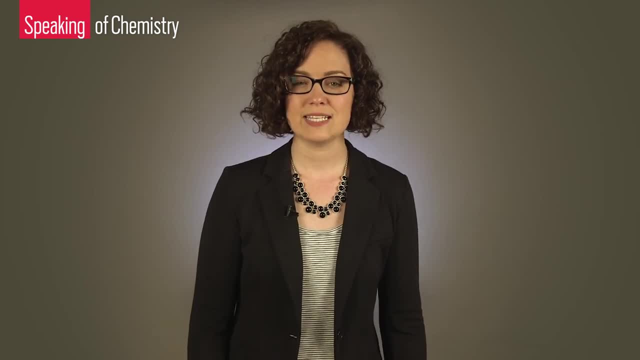 radiation and scintillation light that fit those requirements. He's keeping the exact details a secret for now. We do know the organic scintillator Yeh chose is commercially available, but that doesn't mean this is an easy project. I mean when I first called a chemical company and said, all right, do you have this chemical? 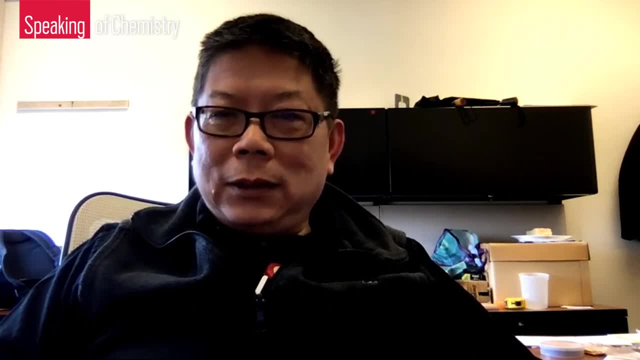 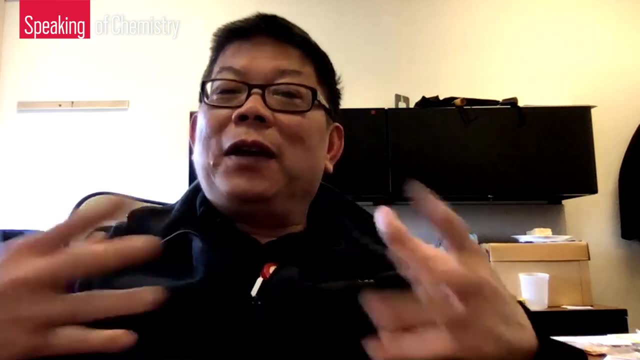 They said, yes, Do you have it in 100 tons? They say: do you mean 100 kilograms Or 100 milligrams? No, no, no, no, no. So this is a very different kind of scale thing we talk about. So this is something very great scientific.